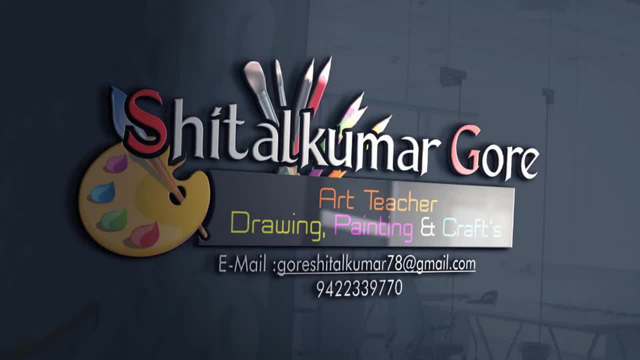 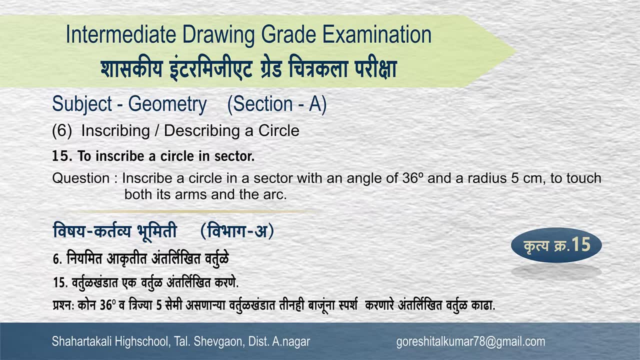 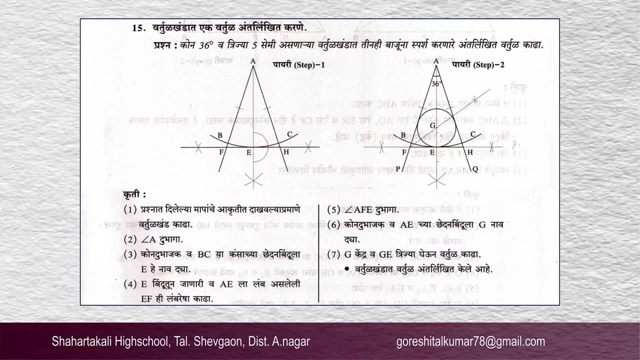 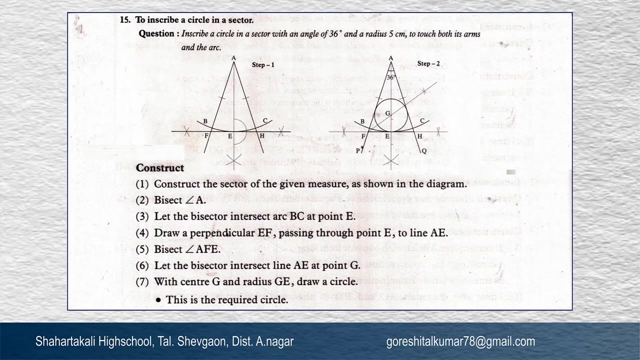 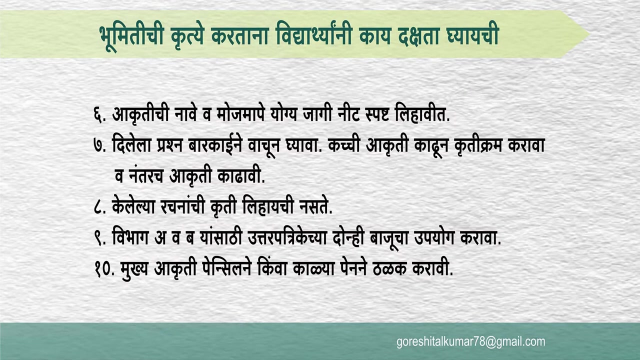 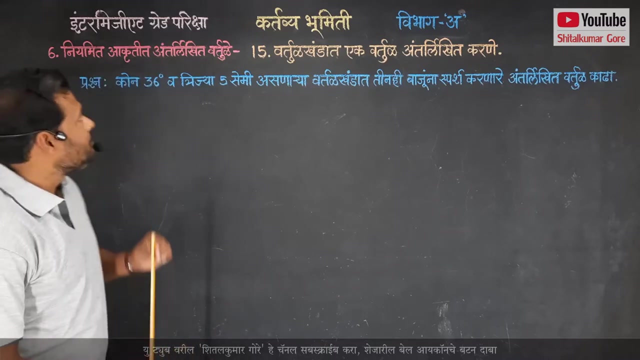 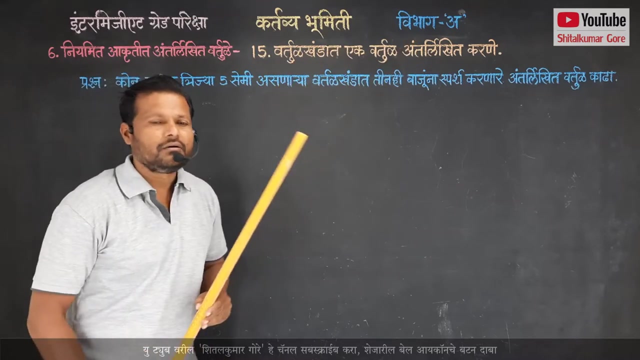 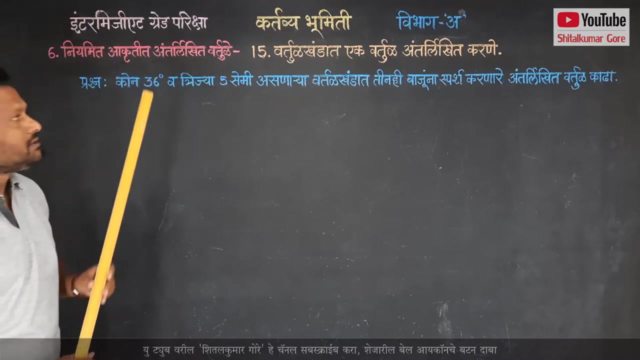 Please subscribe to my channel and press the bell icon to receive notifications when I upload a new video. Thank you for watching Students. in today's section we are going to see an example of the 15th grade film exam, which is written on a regular basis in section A, which is the duty field of the intermediate grade film examiner. 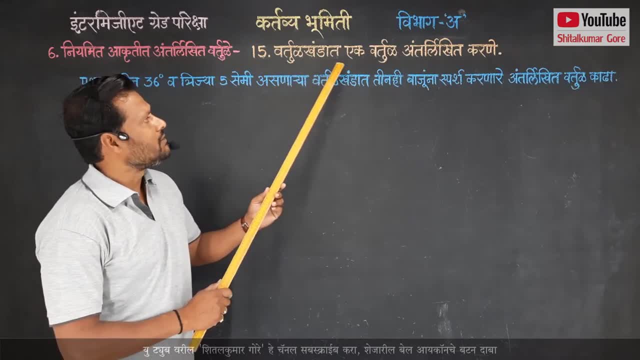 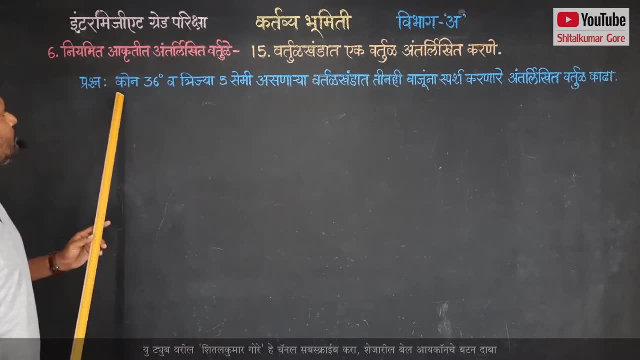 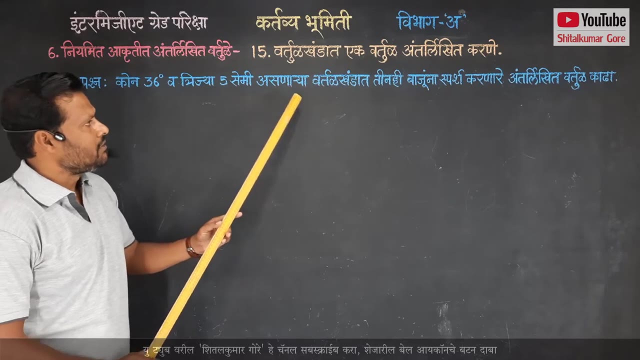 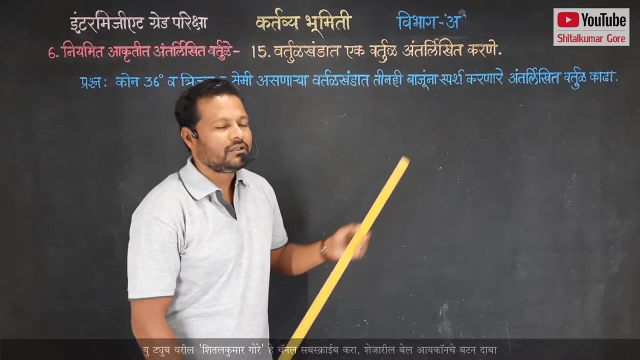 What is the example? In the duty field of the intermediate grade film examiner, one duty field is written. Let's see the question. In the duty field of the 5 cm high film examiner, which is the duty field of the 36th grade film examiner, three duty fields are written. 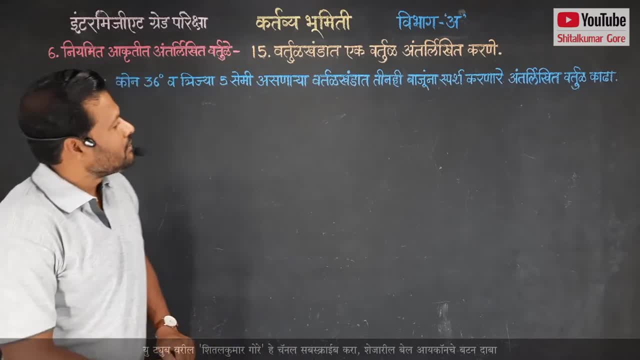 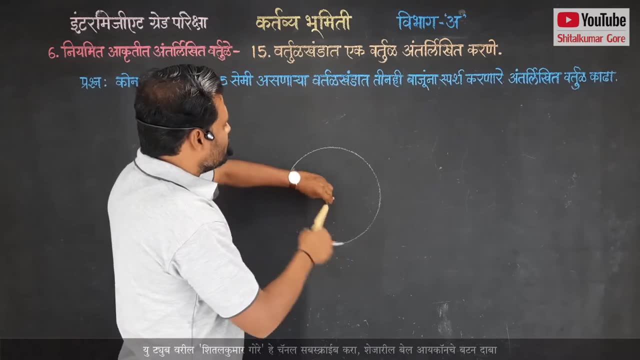 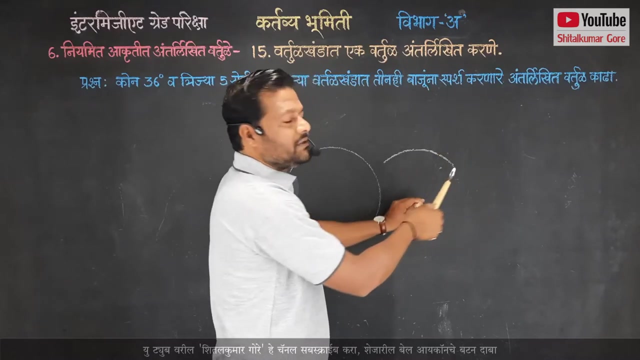 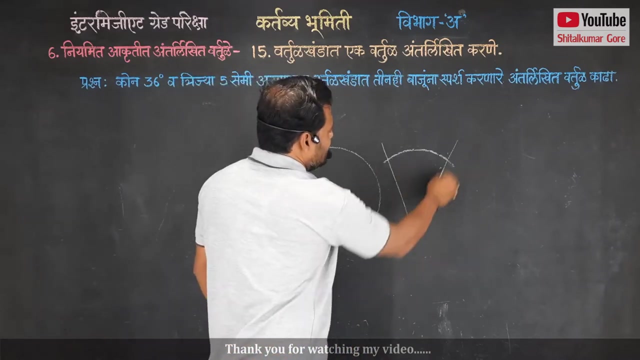 Here we have to remove the duty field. What is the duty field? We've completely removed the duty field, But we have only opened the duty field. The center line which is from here is the duty field. We call the duty field as duty field. 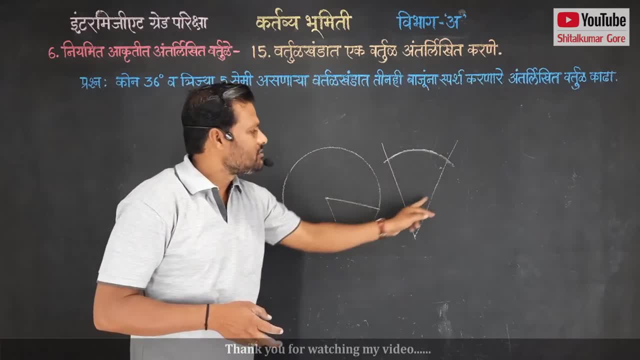 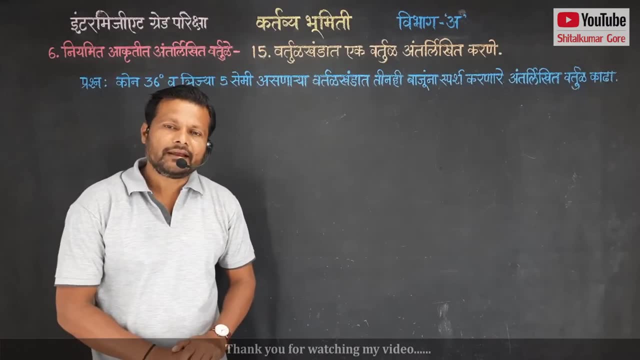 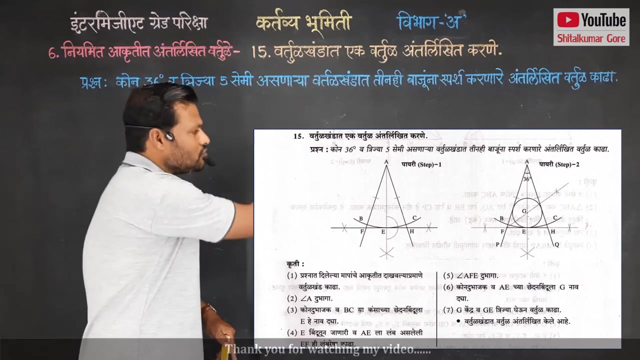 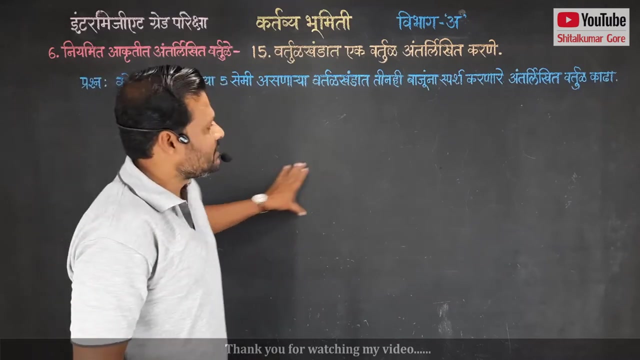 We have to find the point of contact between the two points of contact. Let's start Students. in the grade test book the example is given in the form of a curve. We will draw a curve in a simple manner, as per our own choice. 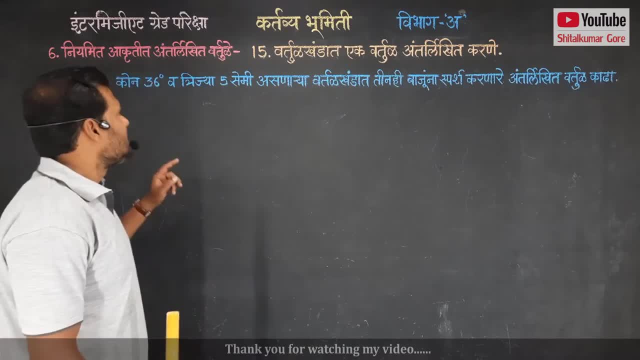 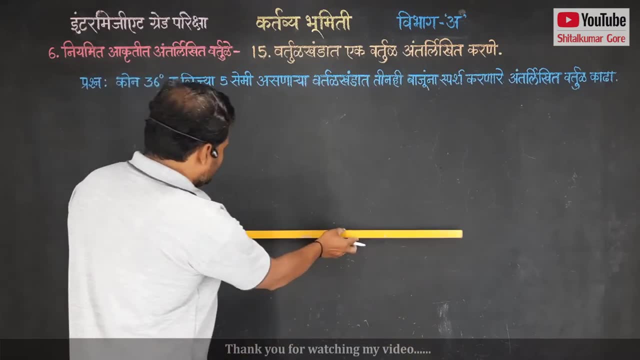 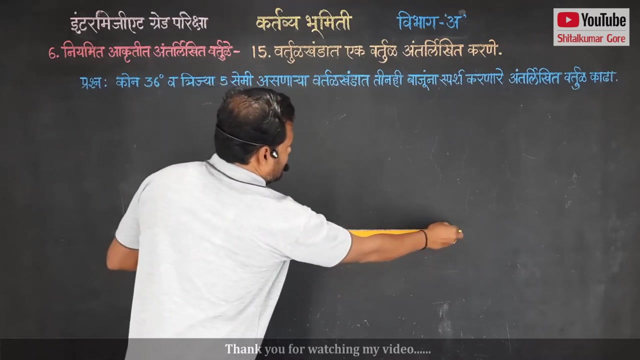 You have to keep that in mind. First of all, we have to draw a cone with a 36 degree angle. For that, first of all, we have to measure the angle of the foot of the cone. Even if the board does not measure it, it will work. 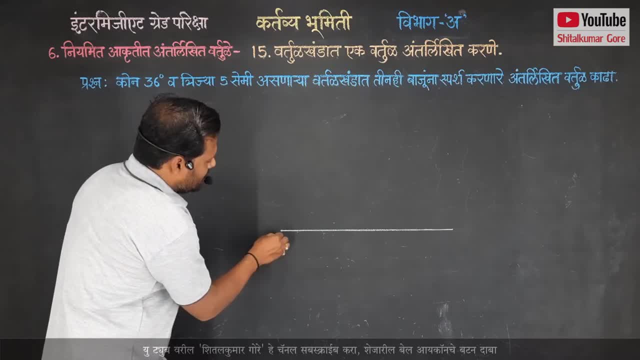 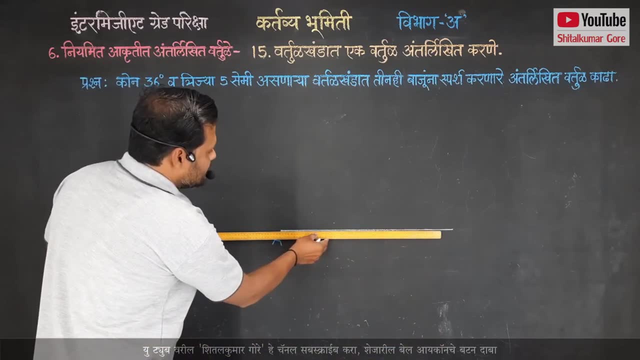 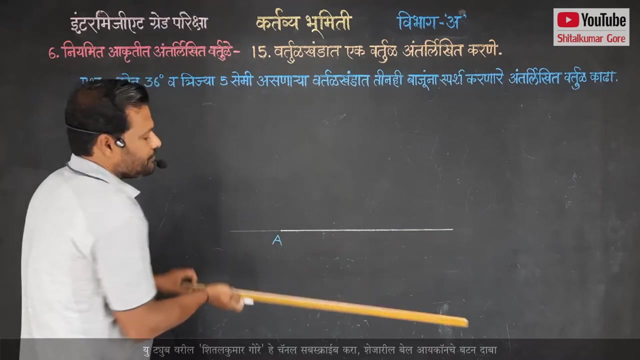 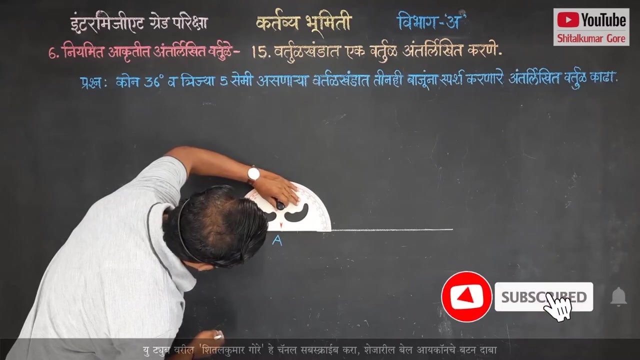 Here let's name the point A. After that this line: here we are increasing the angle a little on the left side because we have to put a cone meter there In this way: put a cone meter on point A And. 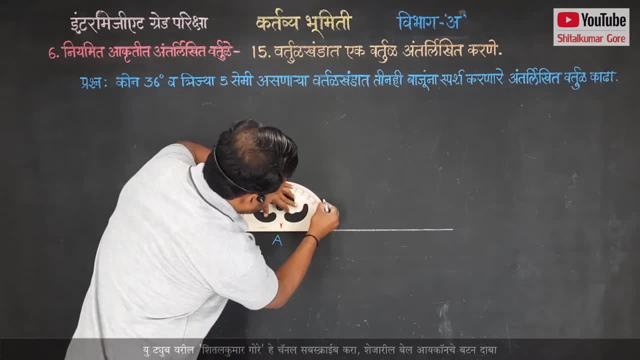 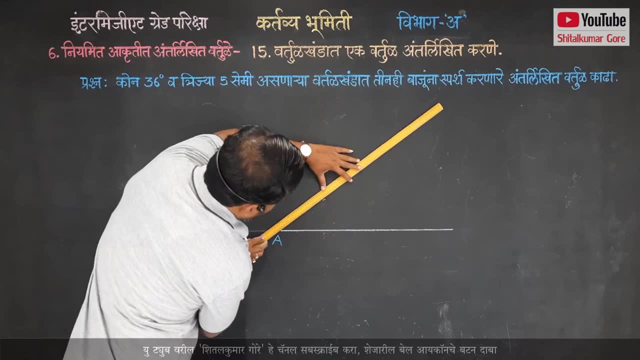 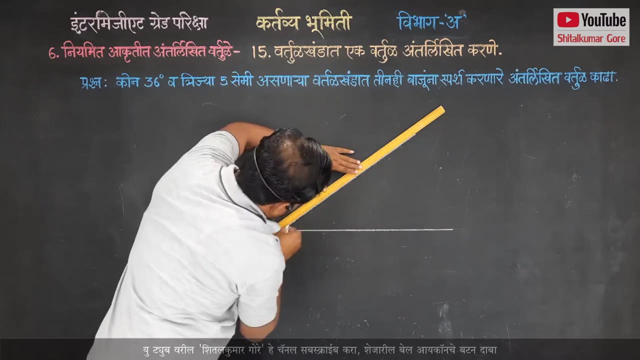 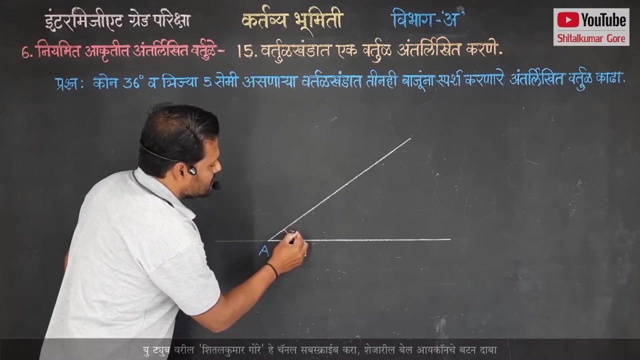 10,, 20,, 30,, 35 and this 36 degree angle cone we have drawn here. We have taken that point, that point and this point together In this way. After that, we have drawn a cone of 36 degree angle. 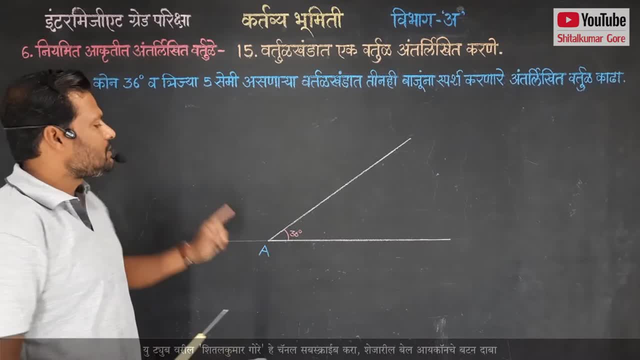 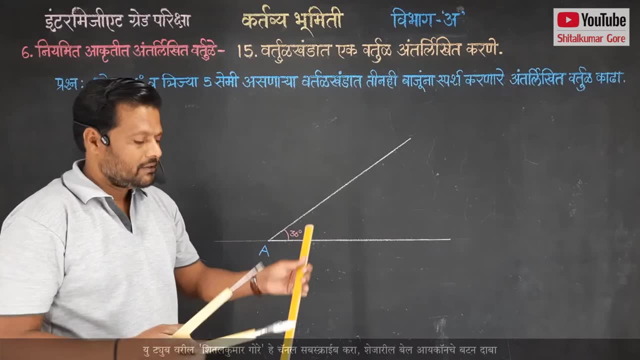 We have to measure the angle. Here we have drawn a cone of 36 degree angle. Now we have to draw a curve above the 5 cm distance. For that, by measuring, we are taking a 5 cm distance in the compass. 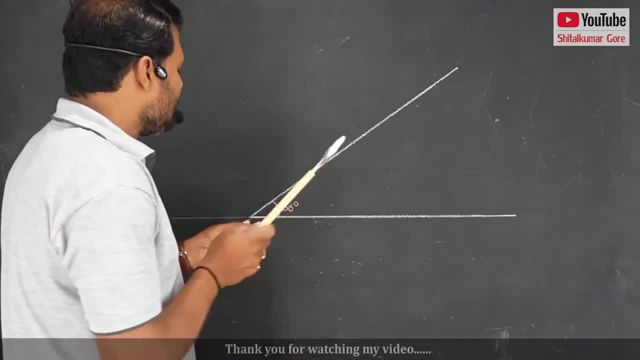 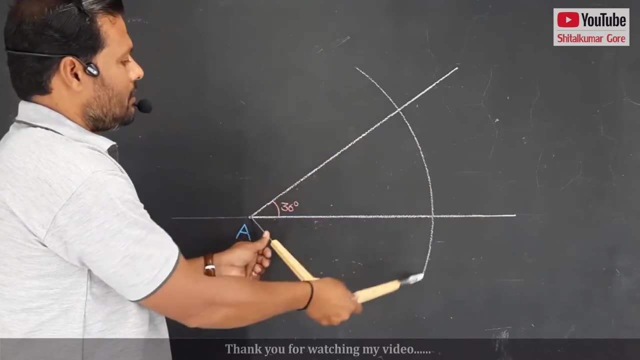 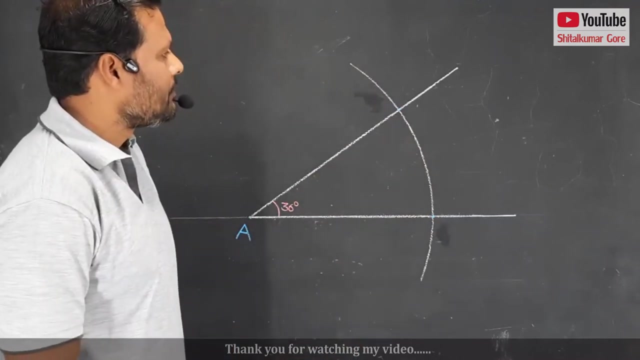 We have taken a 5 cm distance in the compass And we have drawn a cone on this point above the compass. Here we have drawn such a cone. Now the cone above is ready, We have given it the name B and 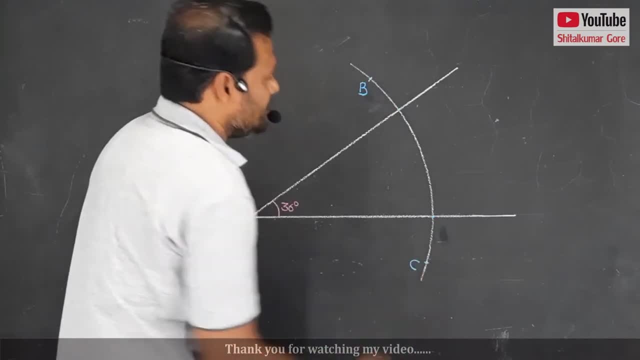 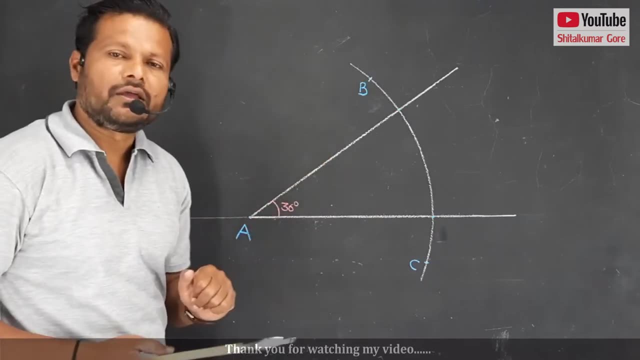 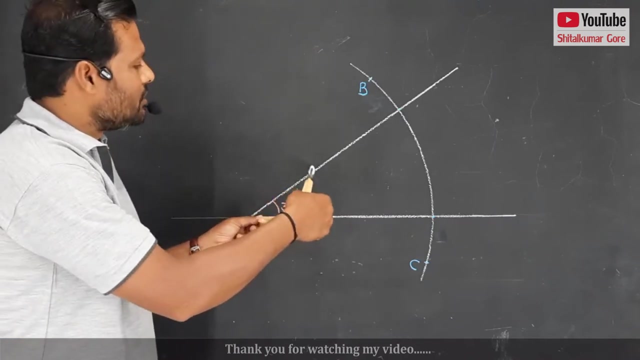 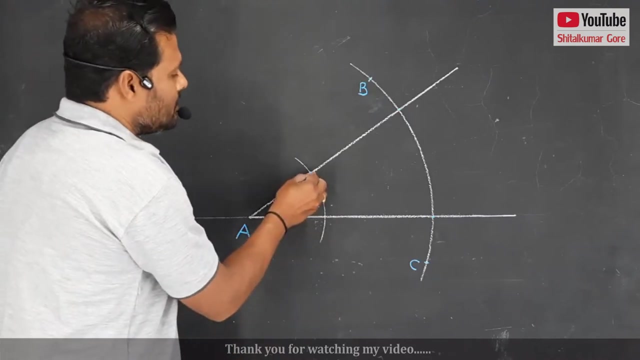 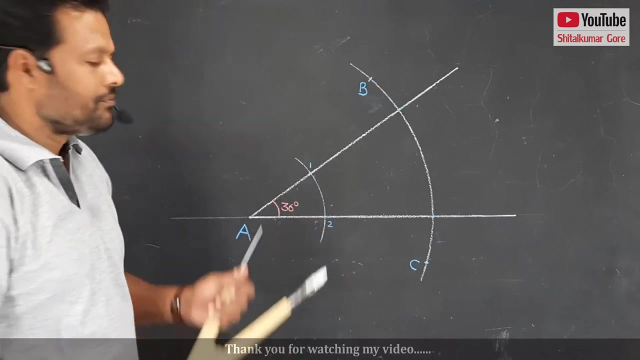 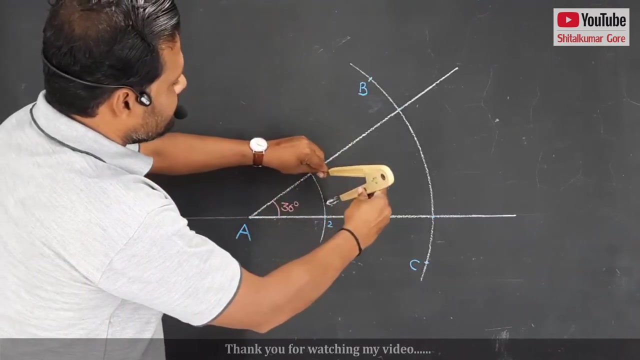 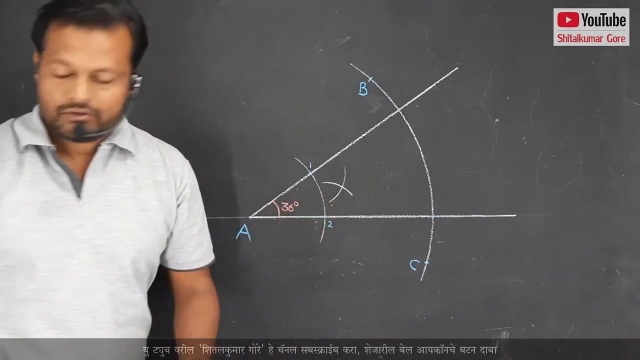 here we have given the name C After that. what we want to measure is the cone of 36 degrees, means we are going to measure it manually. One point spectrometer on the compass. The first point is connected to the second point, the first point is connected to the first point and the second point is connected to the second point. 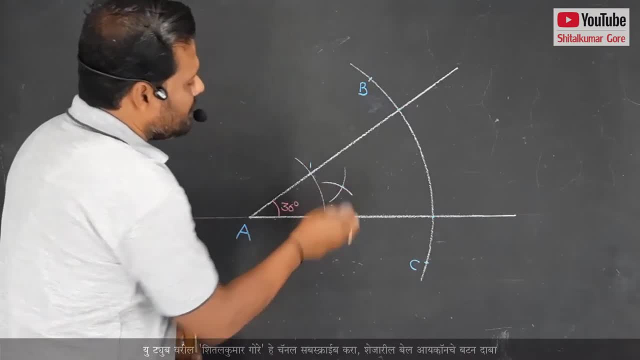 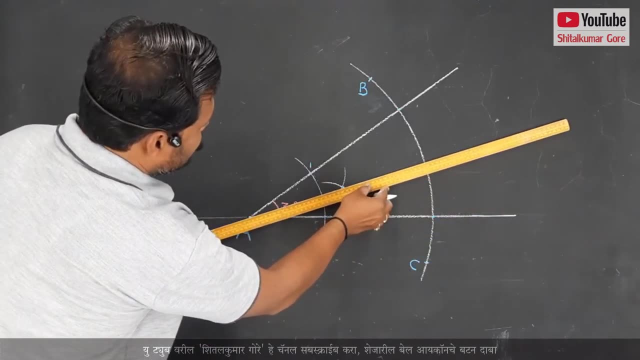 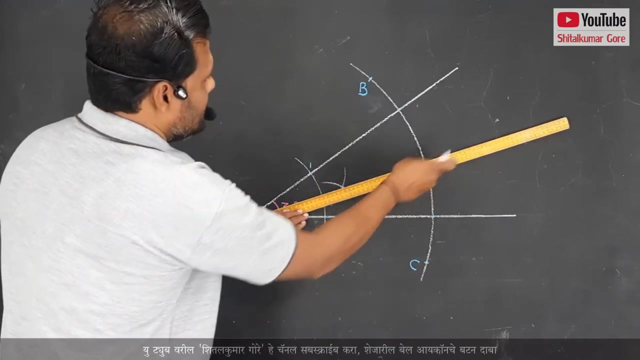 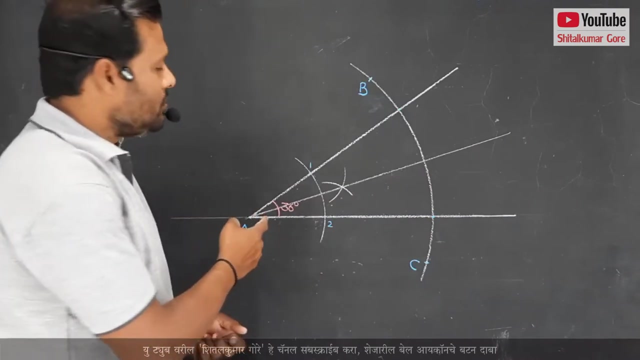 Here the two points are connected to each other. The first point is connected to the second point and the second point is connected to the second point And this line is connected to the second point From this point. which line is connected to the second point? 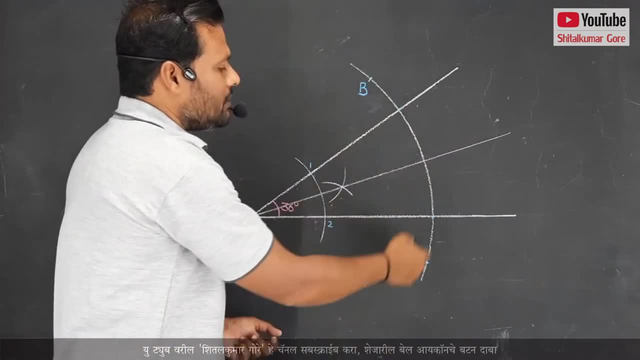 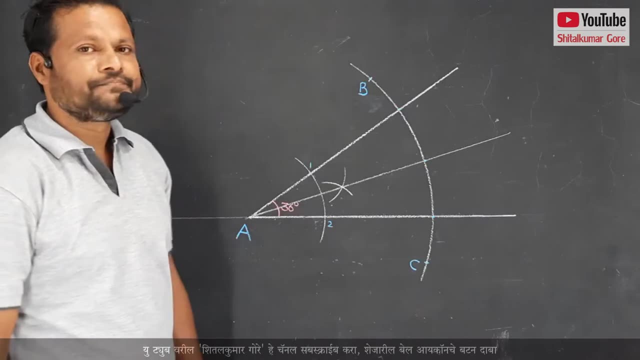 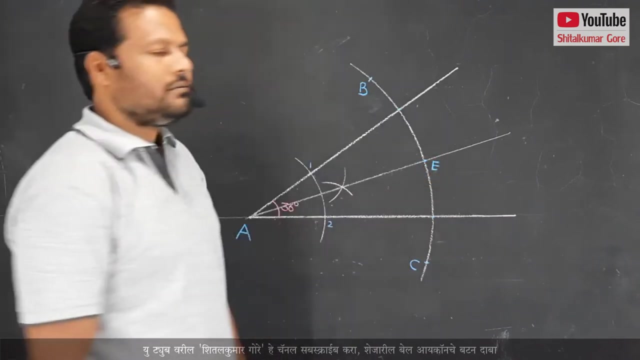 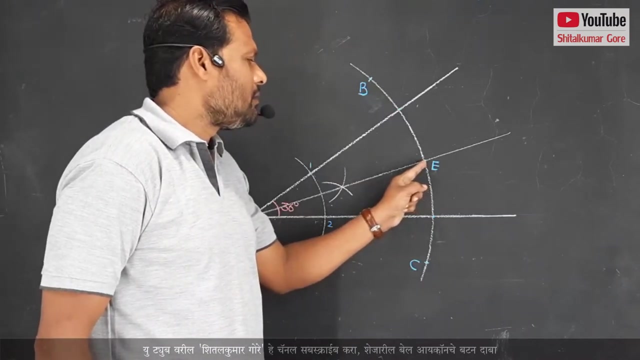 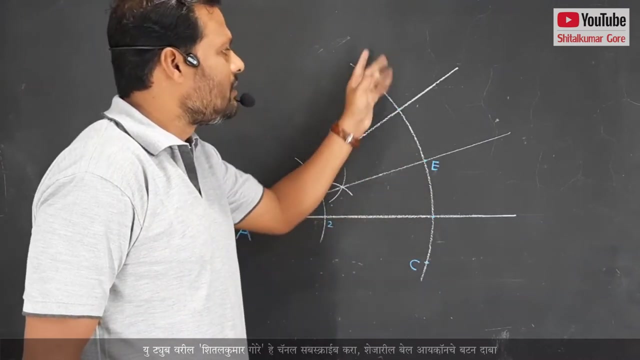 This is the line brought to this other end of the line, that points are connected to the top bound point And the point named e, Now the point going through this point. We have to draw a line here that will touch the cone. 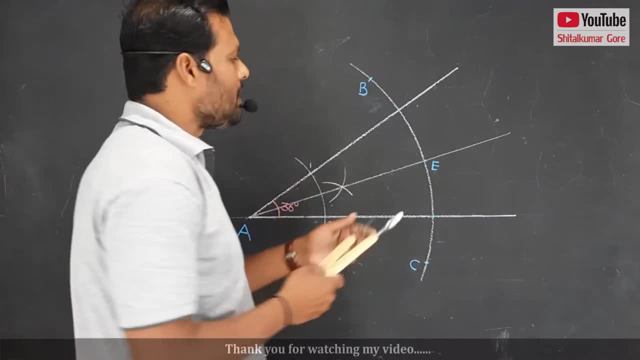 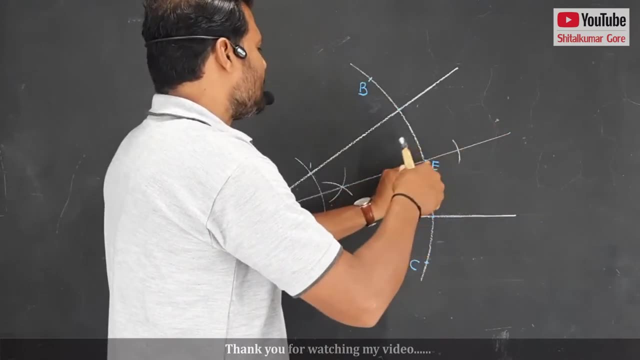 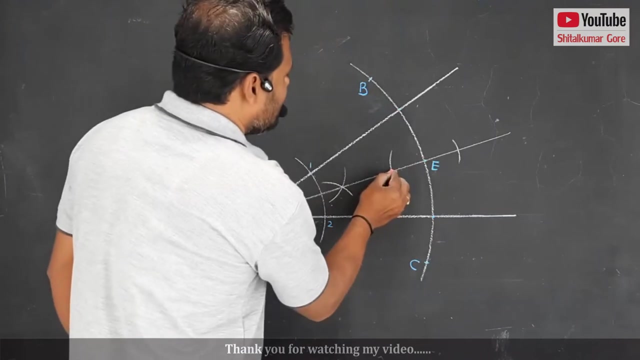 For that we have to keep the point of the compass on this point, And we have made two cones like this by taking the difference in the compass. Wow, Even though the names are not given here, it works. But for your knowledge, what I am doing here is: 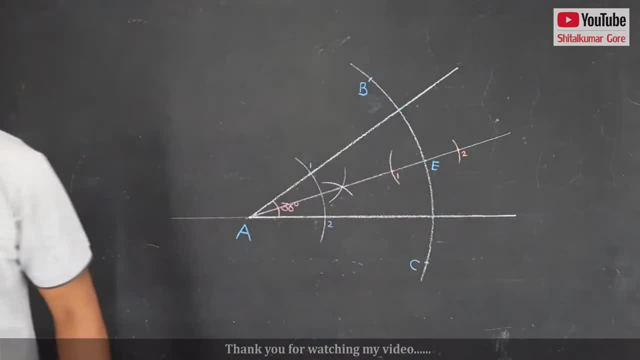 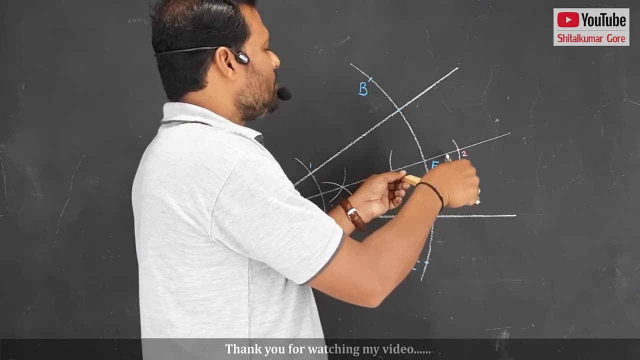 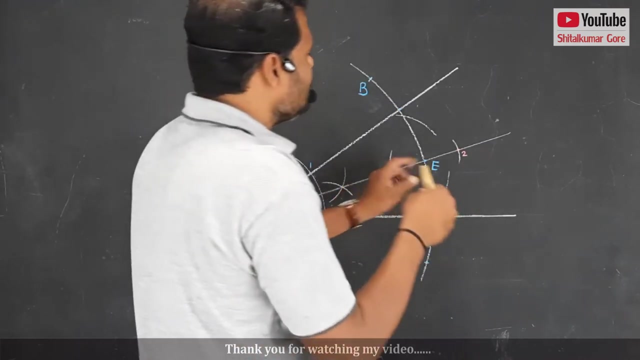 I am drawing 1 and 2 on the compass. On the point of the first compass, we have taken the point of the compass. we have taken a greater distance than the compass. we have drawn a cone at the top and a cone at the bottom. 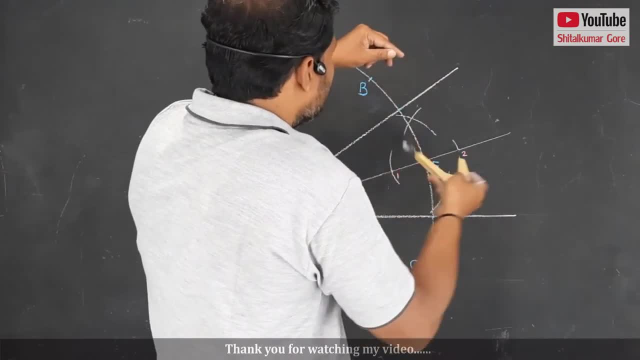 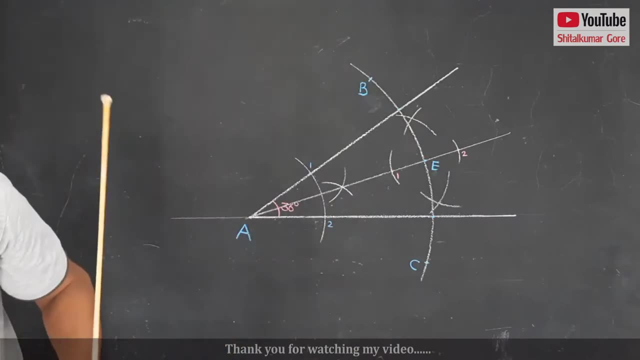 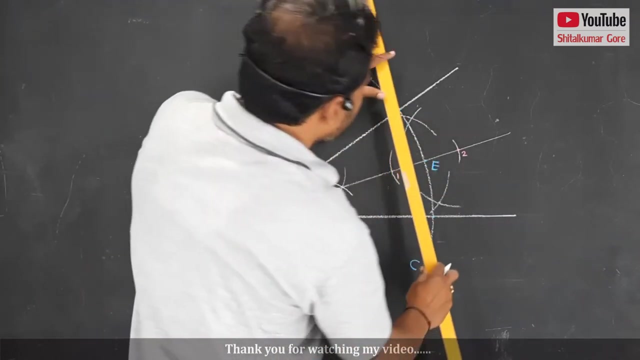 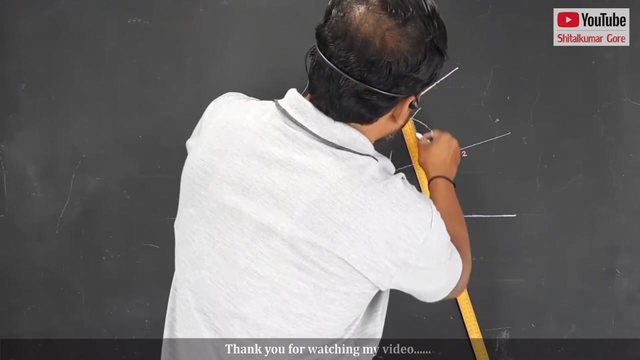 After that, we have drawn a cone at the bottom on the second compass. we have drawn a cone at the second compass. we have broken both the cones into one. we have drawn a point. we have drawn two points and we have drawn these two points in a very accurate manner. 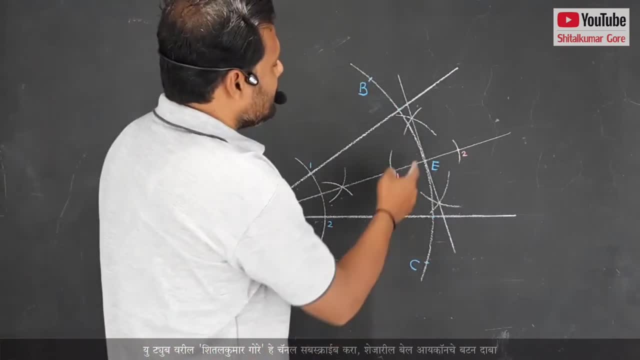 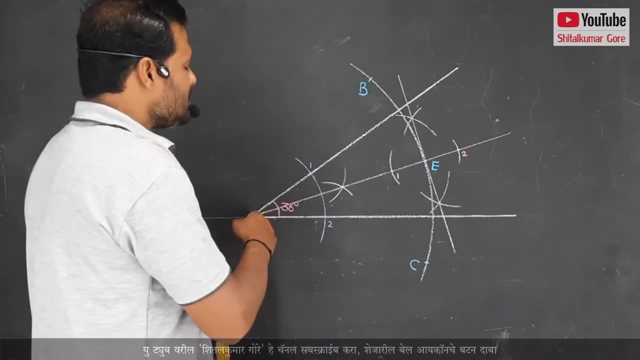 Because of this, we have placed the cone on the top and the cone on the bottom of the compass. This line is drawn here. The line which is drawn is drawn here, at the edge of the 36th- moss cone line. This line is drawn here, at the edge of the 36th- moss cone line. 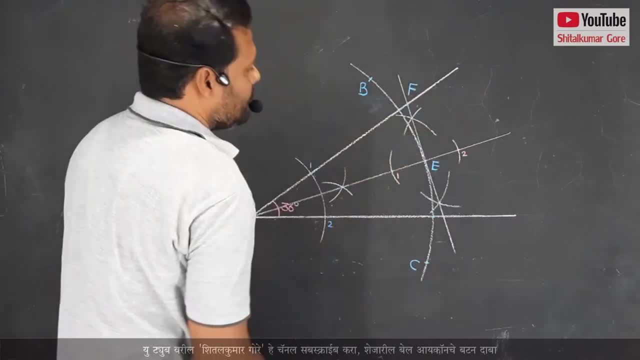 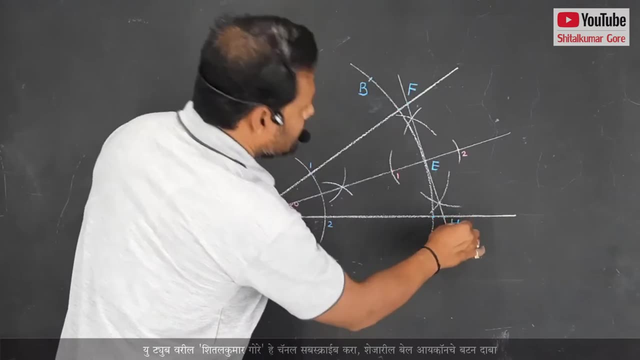 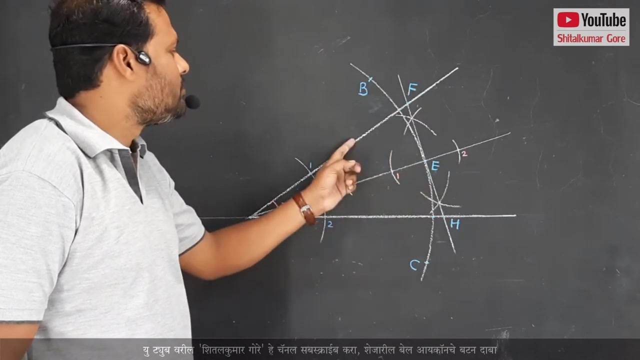 Here I give the name to the point. and here I give the name to the point We have to draw from the top of the compass. like this- and this is the first point of the compass- Like this, touch both the sides of the paper. 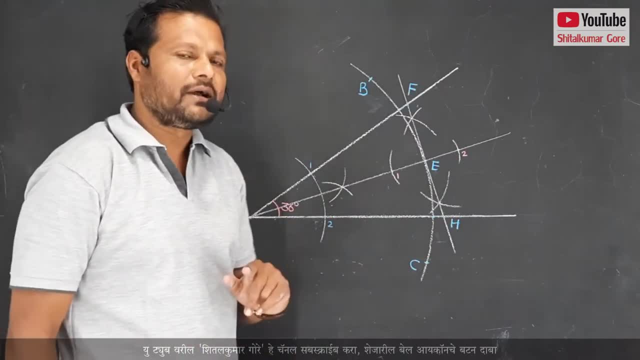 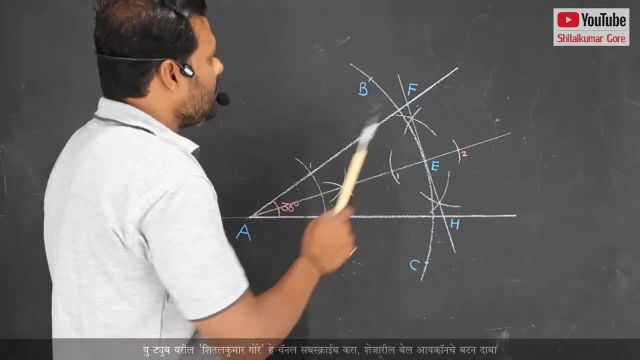 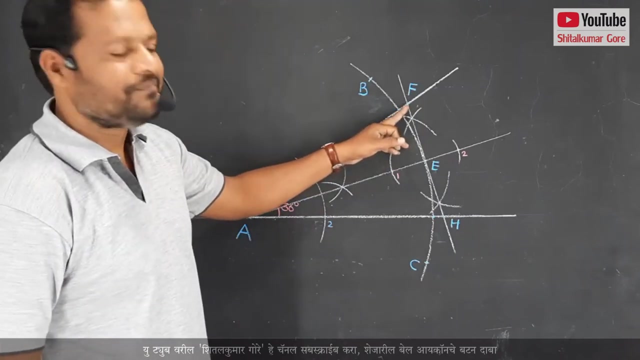 For that. keep in mind Which corner do we want to press. Which corner do we want to press? E, H, A or A, F, E? Will you press this corner? Which corner do you want to press? This corner or this corner? 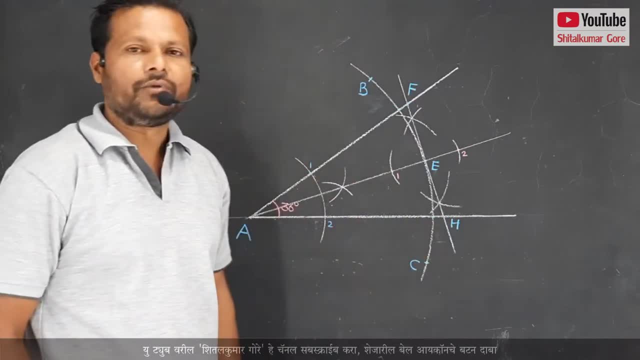 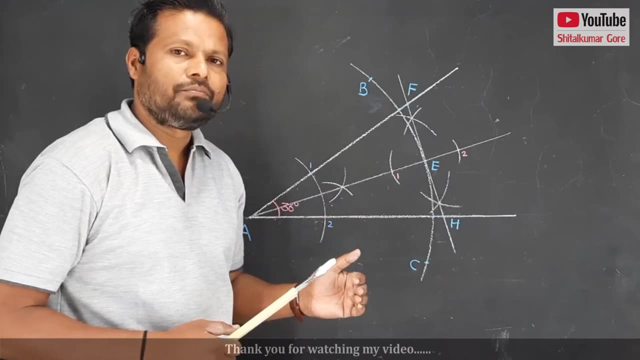 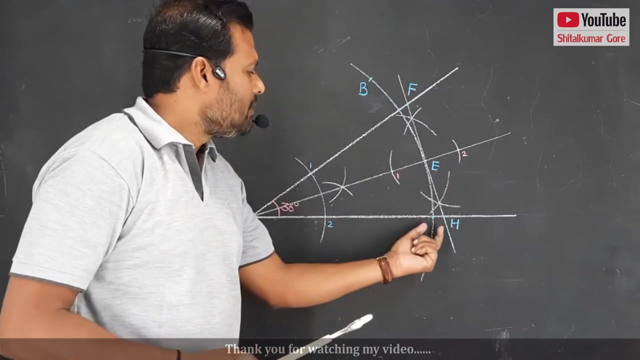 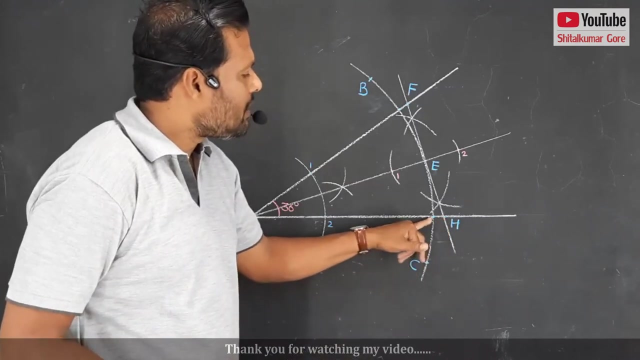 Which corner do you want to press? This corner or this corner? Now, students and friends, Now, as we go ahead in the example, It is an example of the form of a triangle. And look here, Two points are close together, So you can press this point only. 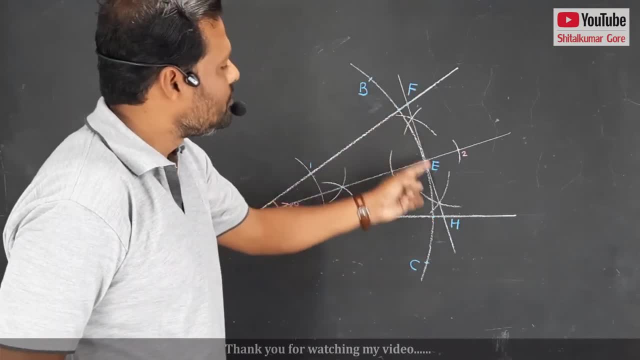 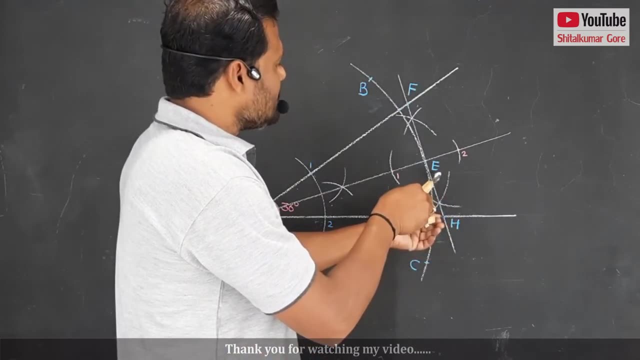 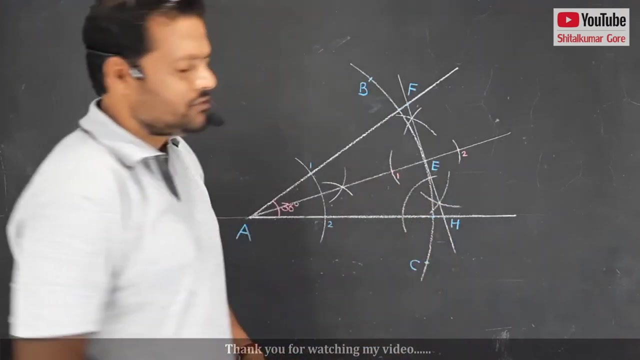 Don't do it like that. The point that we have, So we have to look at this point, That is, we have to place this point on this point. What we have to do here is We have to make a triangle. After making a triangle, You have to. 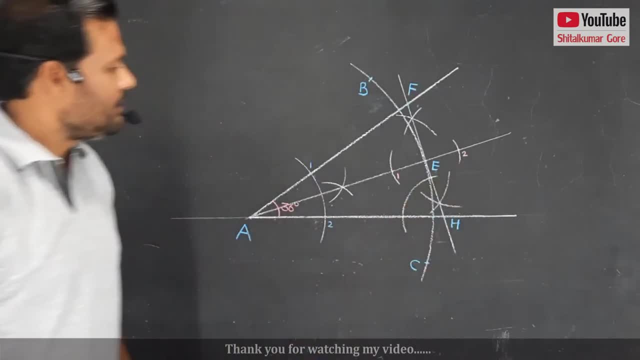 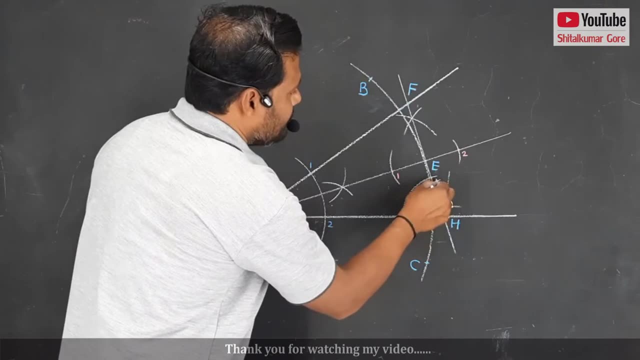 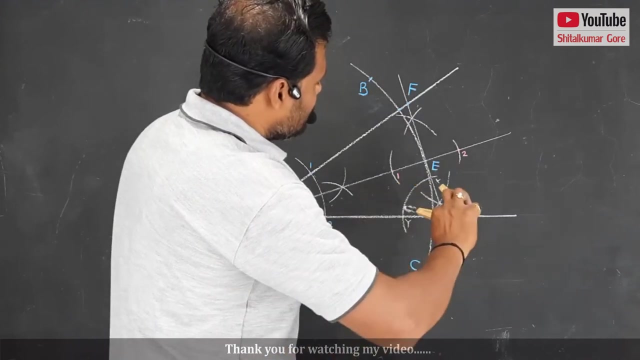 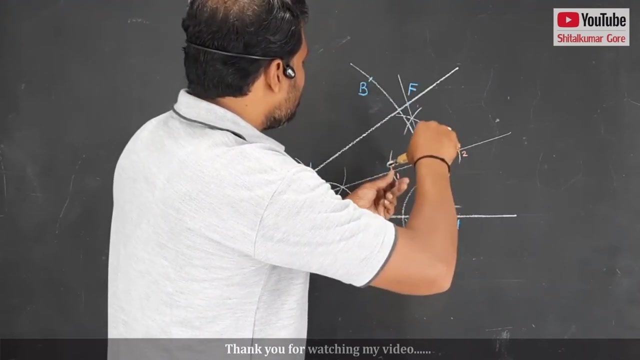 There is a point here And there is a point here. If you feel like you can give a name, Here I will give F And here I will give Y, Like this: The point in triangle is: The point in triangle is: You can see that, You can see that. 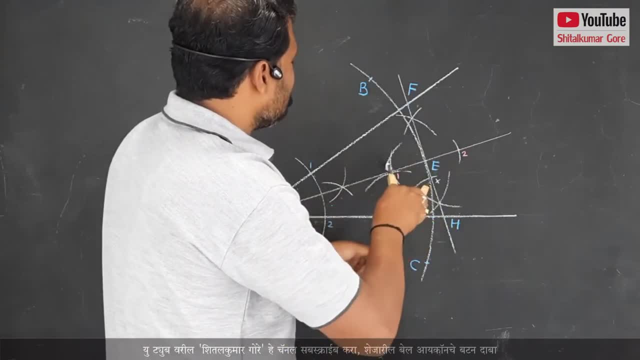 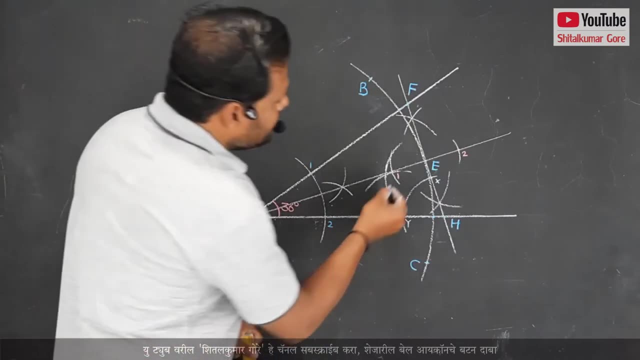 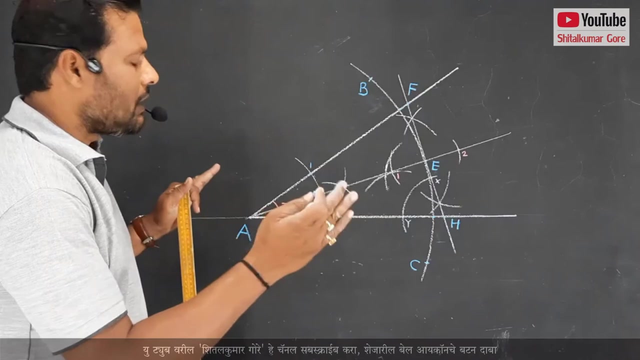 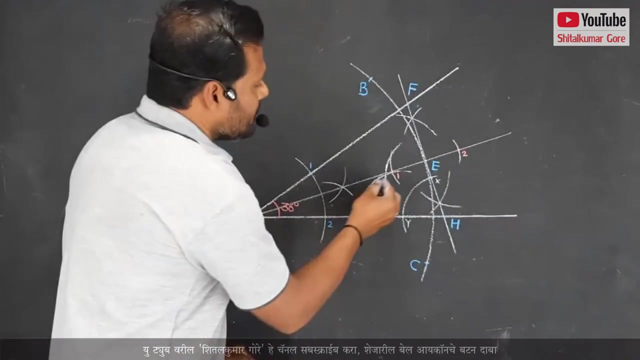 The point is on this side And you have to press here And press here. But if you press this point, I will show you how to do it. Now I will have this big square. Your square will be small, It will be very difficult. So take the point and 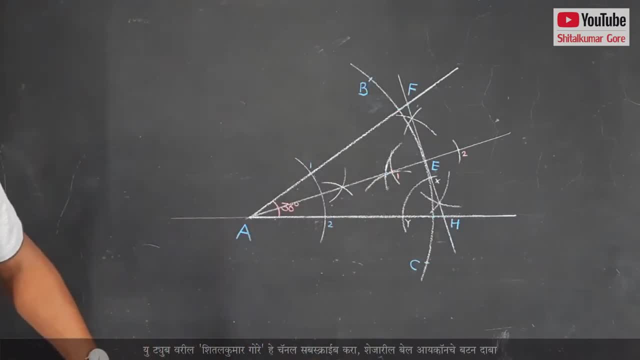 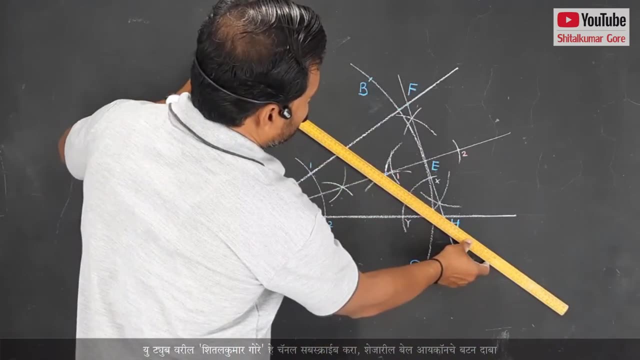 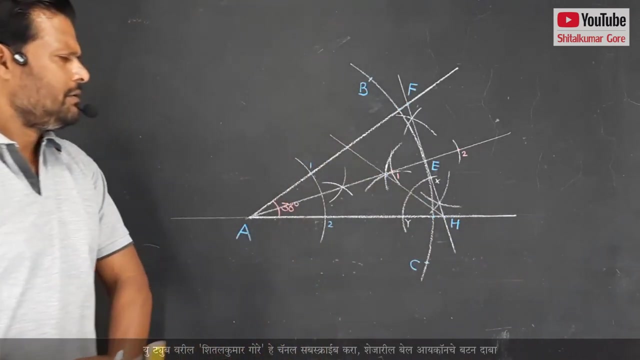 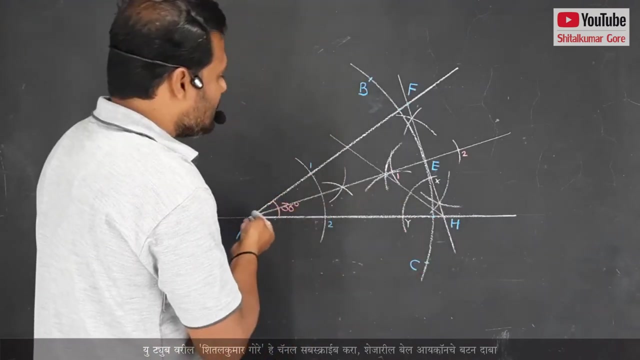 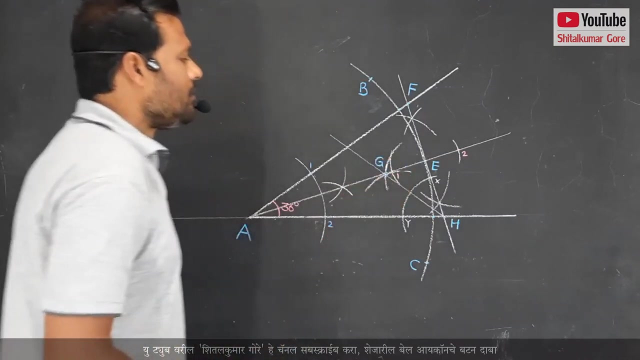 keep in mind which point we have given the name. I have kept the point and I have added this point with the help of line. After dividing this square, we have to subtract the double line. Here we have given the name G. It will be the center point of the top. 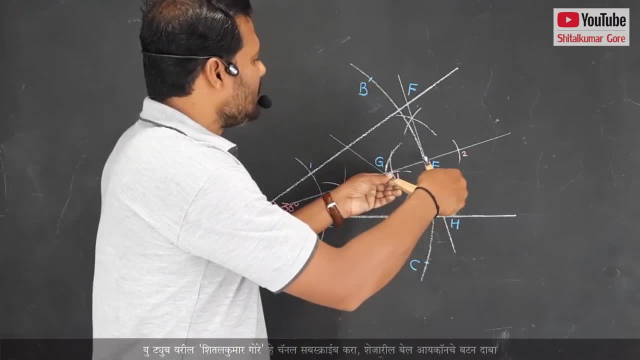 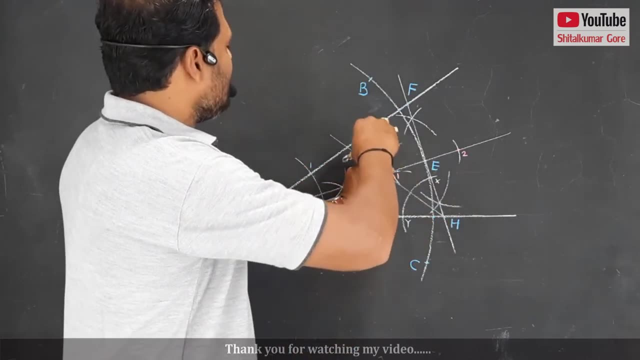 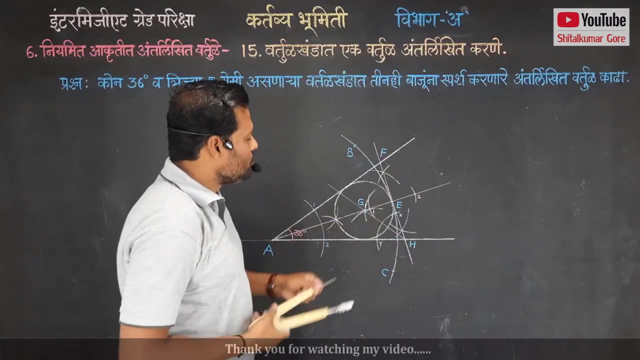 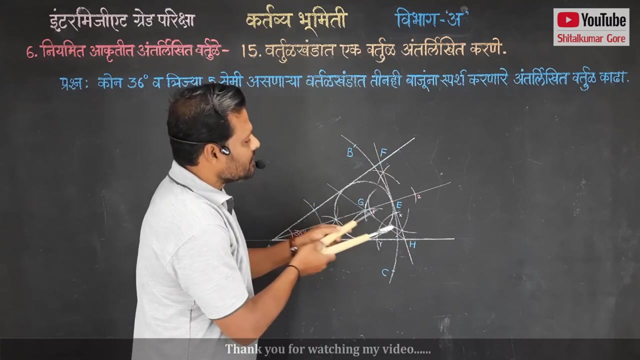 Here we have taken the center point of G And here we have taken the interval, And here we have to subtract the upper line. After subtracting the upper line, keep in mind that this line is directly connected to this line. This line is connected to this line. 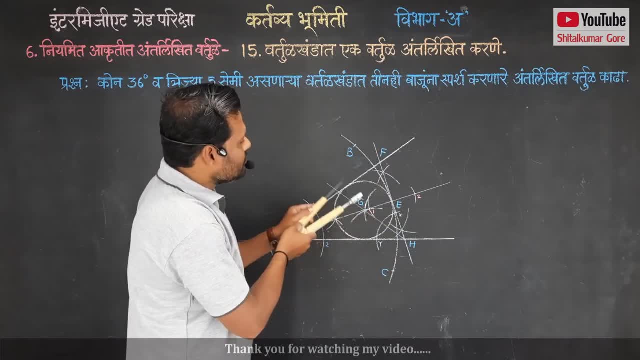 And this line is connected to this line. The upper line has not gone out. This line is connected to this line And this line is connected to this line. So don't go in by touching the line. This will not happen If this happens. 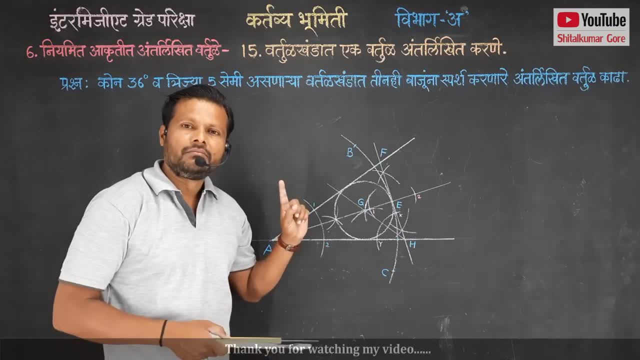 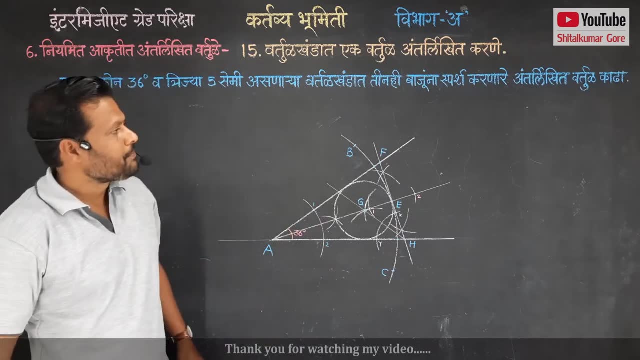 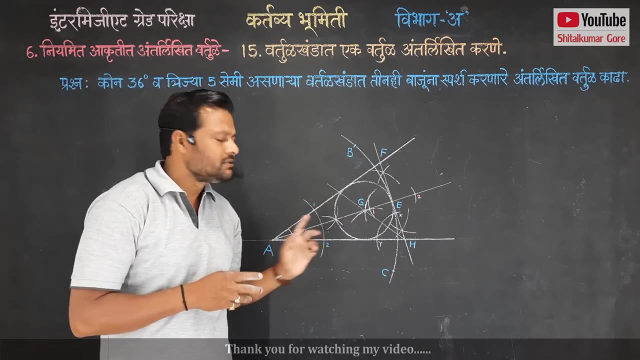 then this example is wrong. This example is a very perfect one. I have left the same example, Friends, while trying to solve this example. change the this interval and solve this example also. Now I am going to present the second example from the previous 14th program.